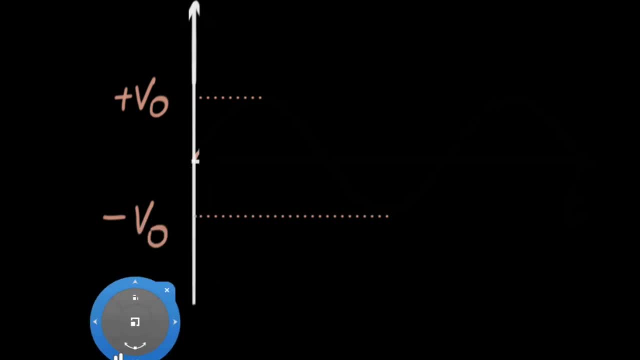 except for this. And now let's see what happens. All right, As I move forward, you can clearly see how the voltage is increasing. You see that voltage increases, increases, reaches positive maximum, decreases, decreases, negative maximum, and so on and so forth. Now I want to make sure that you visualize it. visualize it. 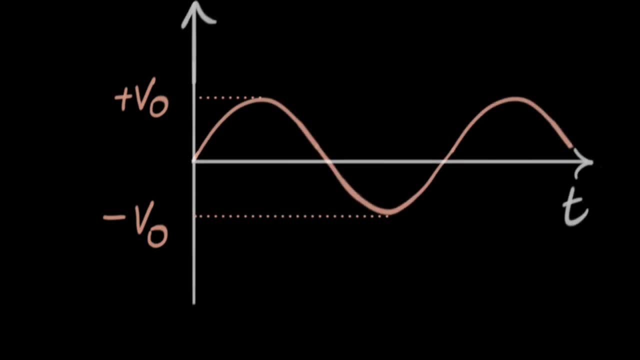 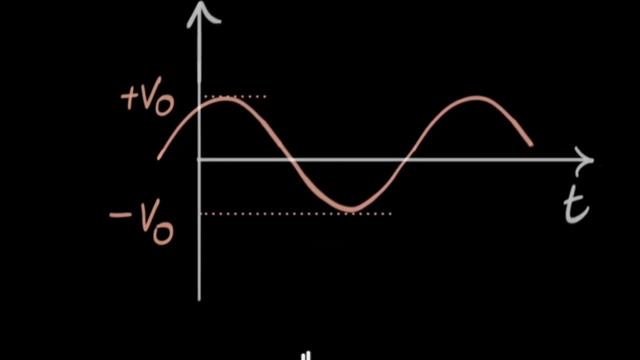 perfectly, And so what I'll do is I'll show you an animation. Instead of moving the time axis forward, I can just move the graph backward, right, And see what happens over here. It's the same thing, right? So let me show you an animation of doing that. So here we go. 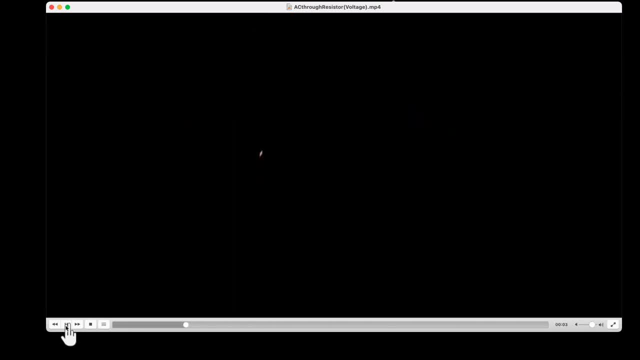 Let's look at that. I'm going to dim everything and you can see voltage going up and down. Can you see that? And we can draw an arrow mark now that represents this oscillation and that the length of this arrow mark represents Vs, the instantaneous value. 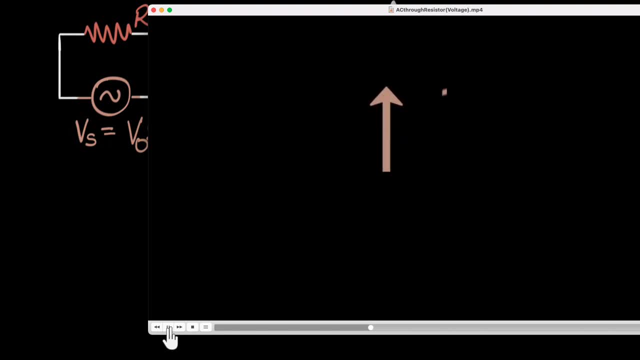 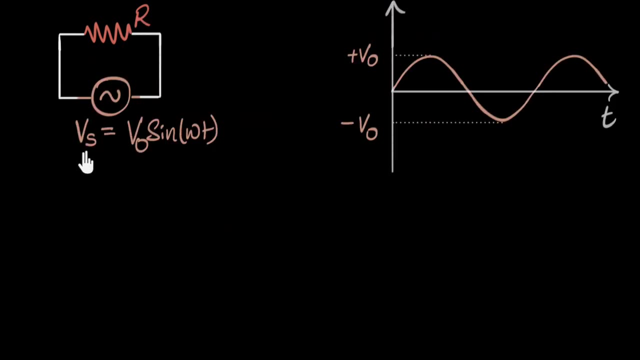 And so right now it's some negative value goes to negative positive maximum, zero negative. maximum positive V0, zero negative V0.. This is how you imagine how it's oscillating and how quickly it oscillates. So let me get rid of this now. And so the number of oscillations per. 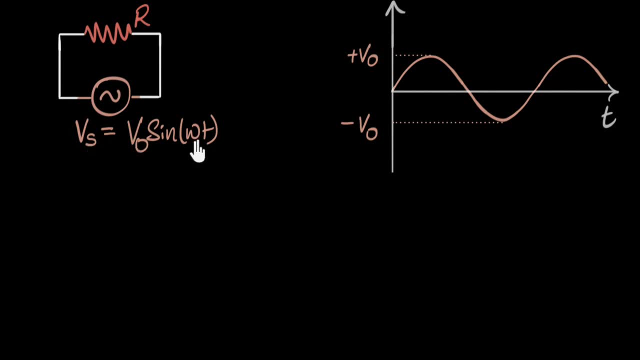 second depend upon this number, omega. Omega gives you the radiance per second, And at first I used to always wonder: what do you mean by radiance? Where is the angle over here? It's oscillations, right. Well, the way to the. 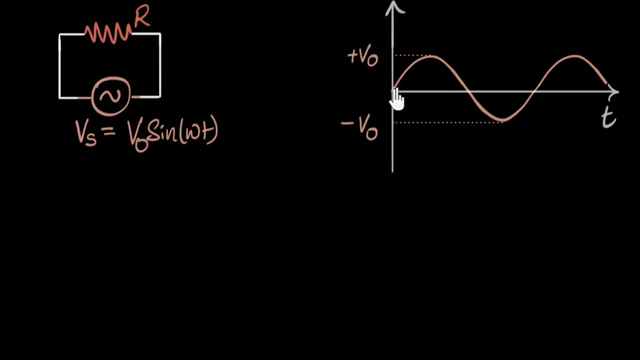 think about it is. you can imagine, one full oscillation corresponds to two pi radians. We imagine it to be like a full circle, and we'll talk more about that in the future, And so it's quite. it's called a phase angle because not real angle. Okay, But anyways. 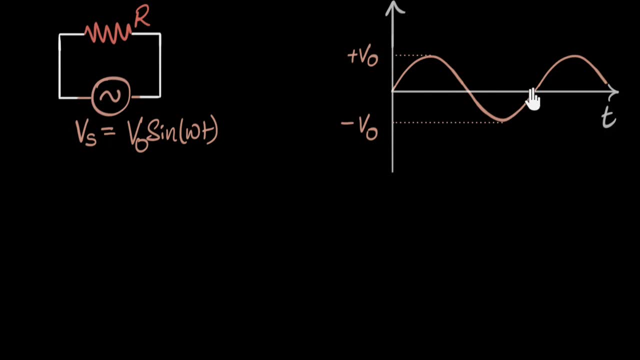 let's not worry too much about that. Um so, one full oscillation equals two pi radians. So if we had, say, 10 oscillations per second as an example, then that would equal two pi times 10 radians per second. Okay, These are all the recap that I'm doing which you've seen before. 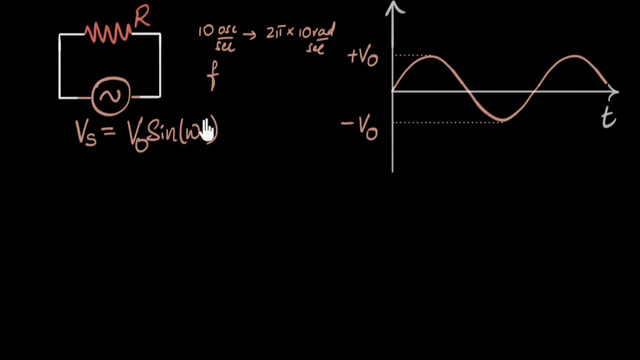 So, in general, if we have F oscillations per second, we can say omega would be two pi F radians per second. And so notice, if you know omega value, you can calculate F. you can divide omega by two pi and calculate F. And so what we want to do now is now that we know about everything, about voltage, 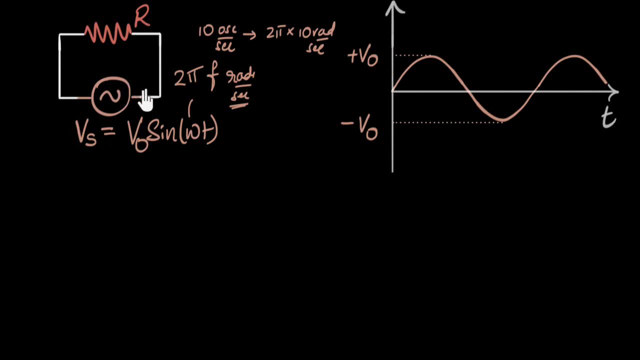 we want to figure out the same thing for current. What's going to look current, look like, what's going to be the graph of that current, how the oscillations would look like, And we want to compare those oscillations with the voltage. 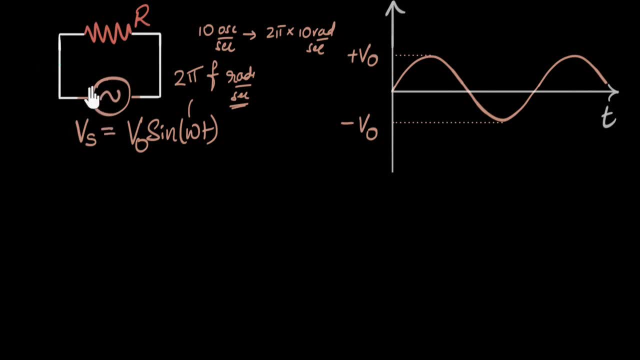 Oscillations. So how do we figure out the current? Well, let's, let's assume the current is flowing, I don't know, maybe this way. And let's say: the current is I. now all we need to do is figure out an expression for current and equation for current. So where do we begin? Well, 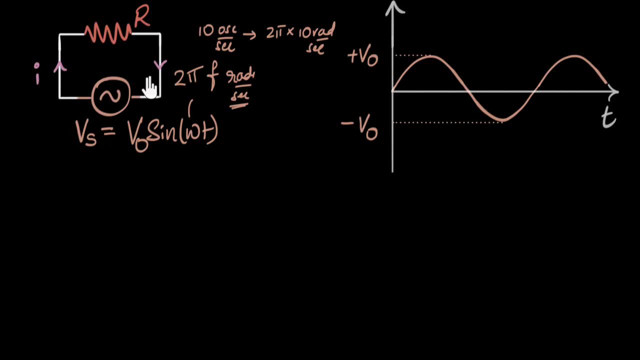 since we only have a resistor in our circuit, we can go for Ohm's law. We can say: whatever is the voltage across the source, same to be the voltage across the resistor, because you're only one element, and then we can use Ohm's law. So it'd be a great idea to pause the video and see if you. 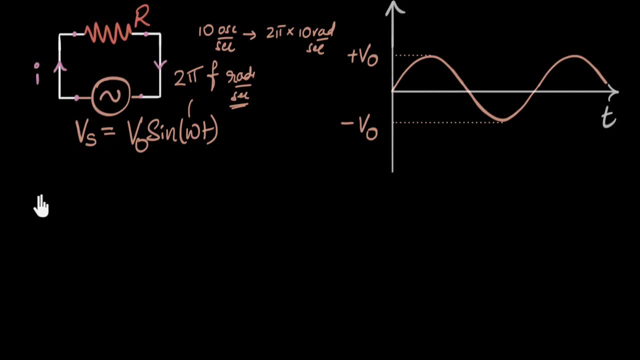 figure out the equation for current yourself, All right. So we can directly say from Ohm's law: the current equals voltage divided by R, So voltage across the resistor divided by the resistance. And we need to be very careful. at least right now there's only one component, but in future. 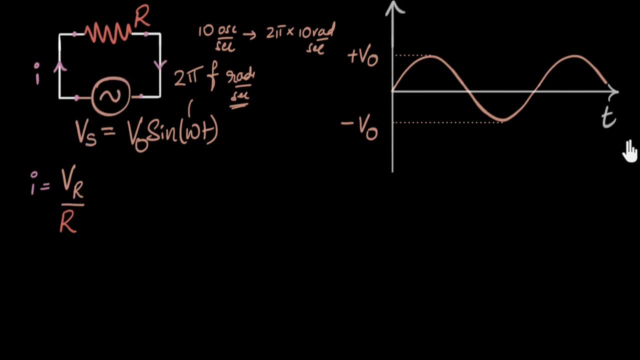 you might have more components. So it's voltage across the resistor divided by R. It's not just any voltage, but in our example, voltage across the resistor happens to be the source voltage, So that divided by R, and this happens because there's only one component. 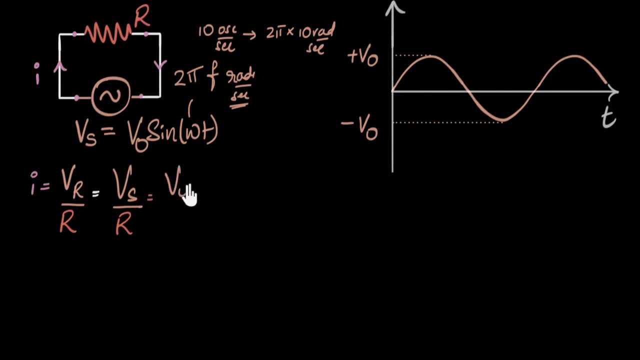 And we know our source voltage is just B naught sine omega t. So our current is just going to be this, divided by R, and tada, we have found our current directly from Ohm's law. And what is the equation saying? The equation says that the current is also oscillating. We also had the same. 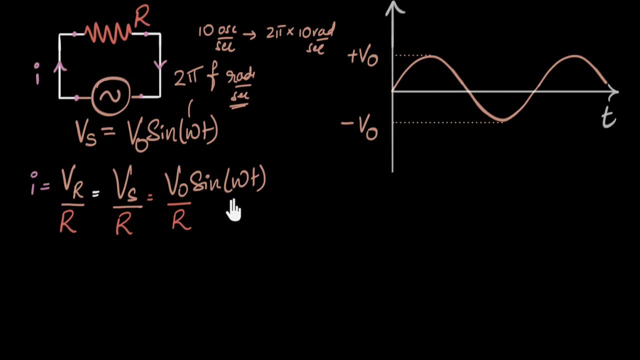 sine function over here, which is not a surprise, not really all that much of a surprise. It also tells us: let's look at the relationship between the two. It also tells us that it's oscillating in sync with voltage. What does that mean? This means when the volt, let's say when the omega t, is zero. 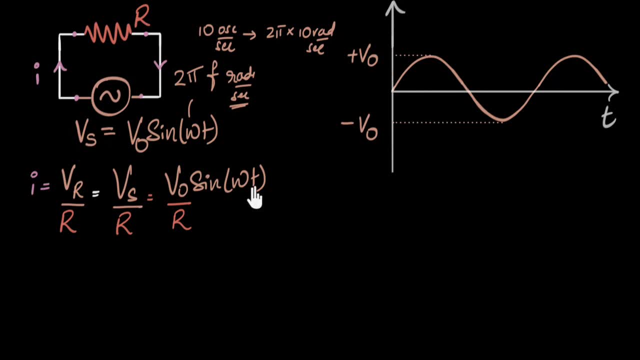 then our vs will also go to zero, because sine zero is zero, And at the same time current will also go to zero. Similarly, when omega t is 90 degrees, our vs goes to maximum. this will also be maximum. current will also go to maximum. So you can see. 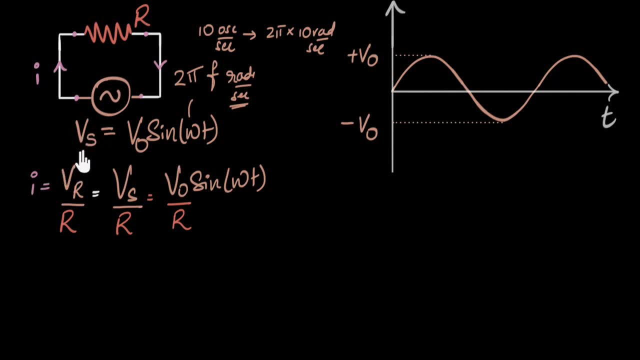 because they have the same function, they'll be oscillating in sync with each other. Does that make sense? And again, that makes sense to me because Ohm's law it says when the voltage is maximum, current should also be maximum. When the voltage goes to zero, current should also. 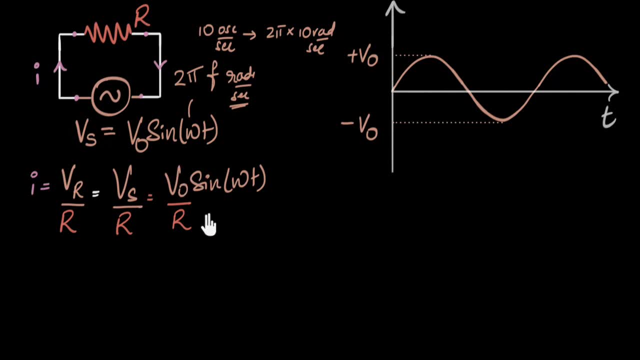 be zero. So that kind of makes sense. It's nice. And what does this number represent? V0 divided by R, that represents our maximum current, And we can call that I0 now And again. it's not a very much. 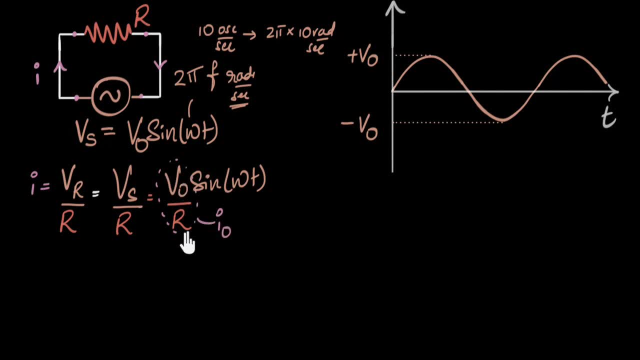 you know, it's not a big surprise- that the maximum current is just the maximum voltage divided by R. So now it would be a great idea for you to pause the video and see what the graph for current is going to be. So can you visualize or try drawing a graph on top of this itself? current. 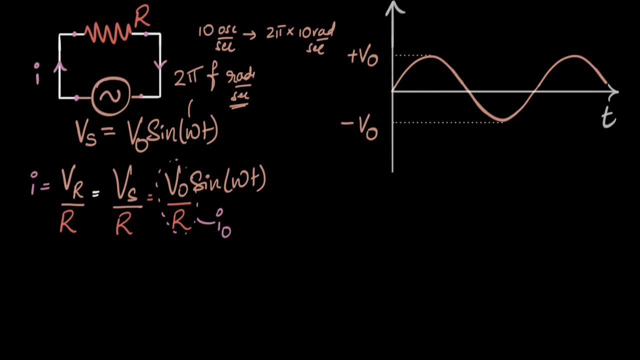 graph. pause the video and see if you can draw it yourself. Okay, let's do this. This is what it would look like. And so now this peak value represents the positive I0 and this would represent negative I0.. So this would be our positive I0, this would be our negative I0.. 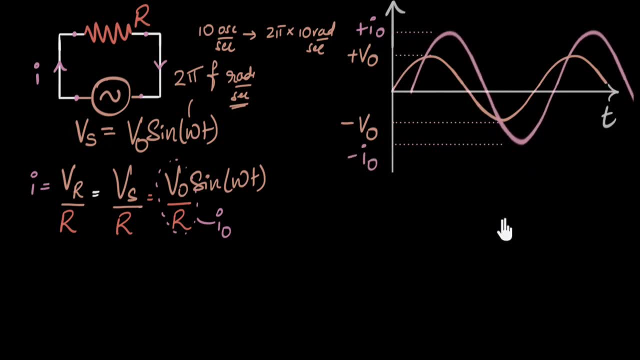 And notice how the graph is. The graph is not shifted like this. The graph is exactly this way because they're in sync. they go to zero together, maximum together, zero together, minimum together, and so on. And again, if you want to visualize this, we can dim everything. 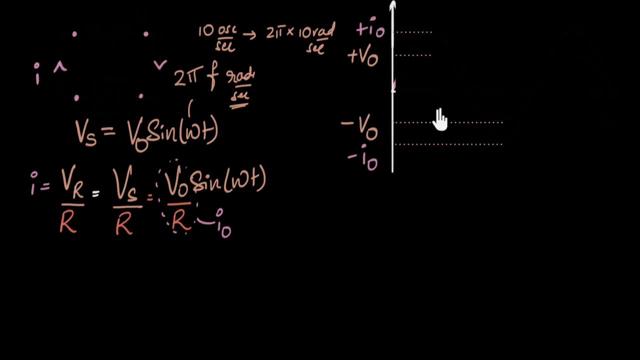 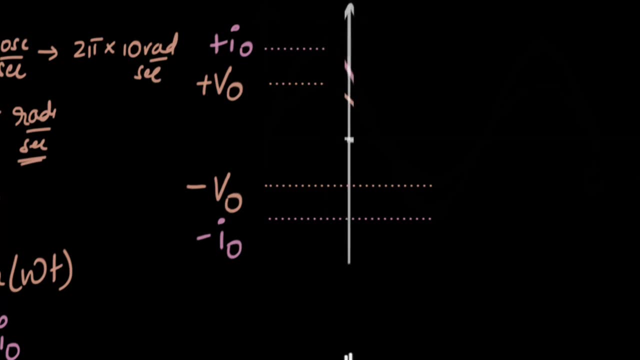 and we can move our time axis forward. So just concentrate over here. Okay, if you move the time axis forward, see how they oscillate. They both go up together, they both go to zero together, both go to the negative maximum together, and so on and so forth. That's how you visualize. 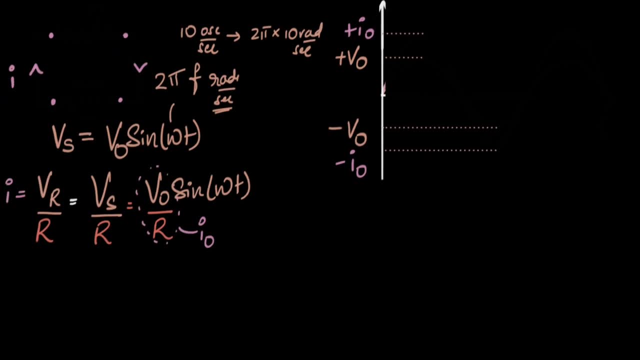 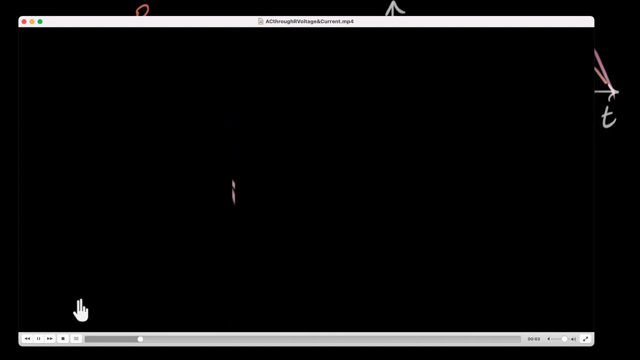 They're oscillating in sync with each other. And again I have an animation for you. We can move the graphs to the left and we can decrease it, and you can use the same thing. And again we can draw an arrow mark, because it makes it easier to visualize with an arrow mark. 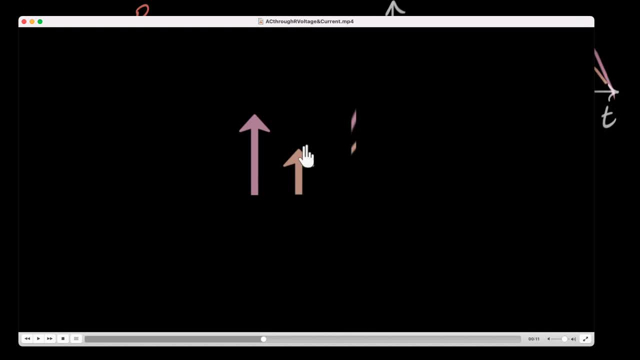 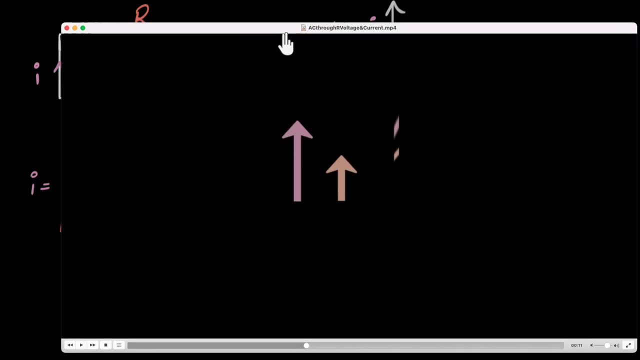 And you see they're both oscillating together. This represent the length of, this represents vs, And the length of this arrow mark now represents the current I. Okay, And so it goes to maximum, zero, minimum, and so on and so forth. I have one question for. 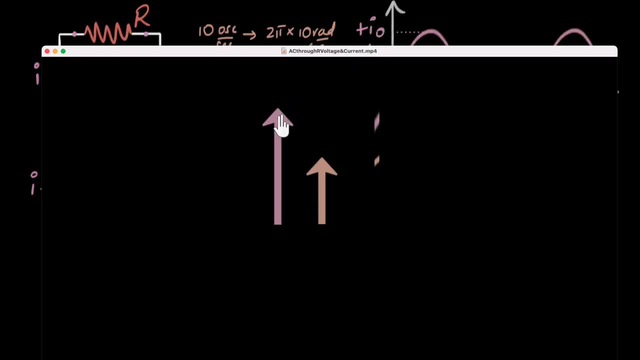 you And I want you to think about it. I have drawn the current length to be bigger than the voltage length, or here, Same here currently, and currently maximum to be bigger than voltage maximum. Why? Why is that? Can you pause the video and think a little bit?